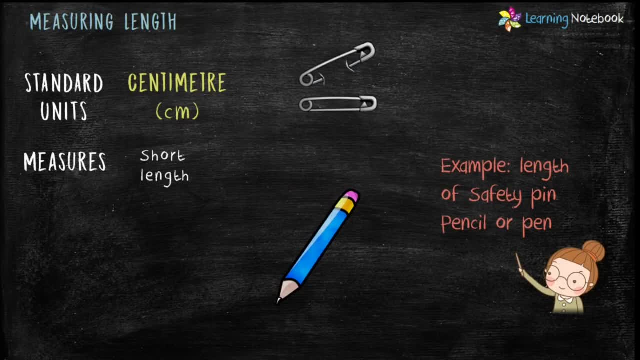 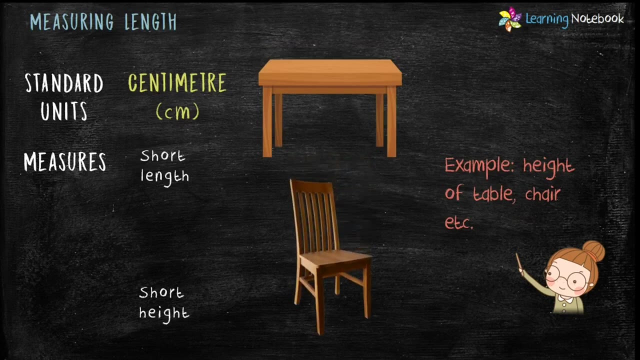 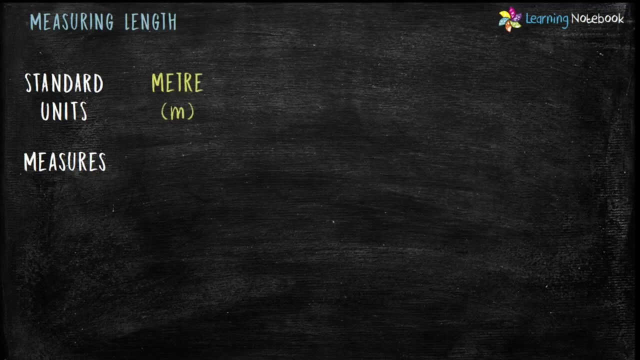 length, For example length of safety pin, length of pencil or length of pen. They are measured in cm. We also use cm to measure short height. For example, height of table table is measured in cm. Next standard unit to measure length is m. In short, m is written. 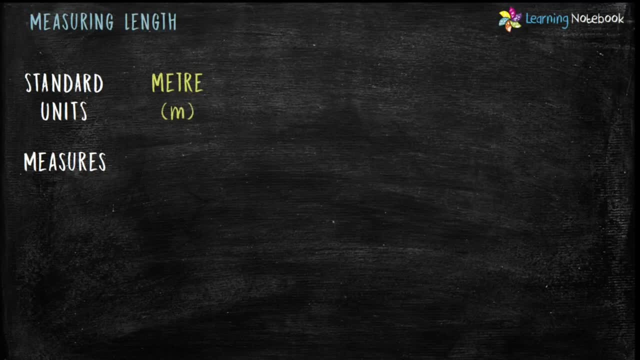 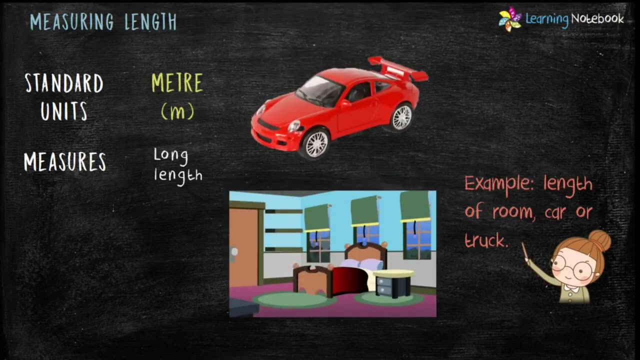 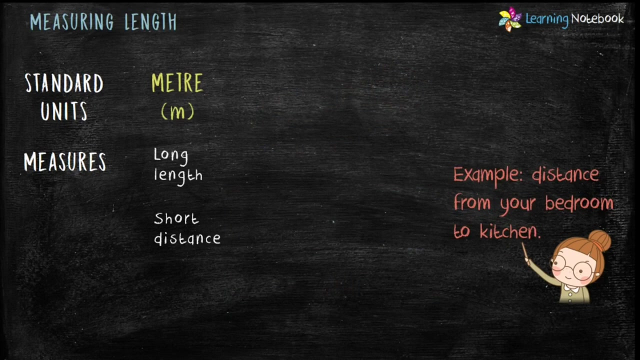 as m. We use m to measure long length, like length of room, length of car or length of truck. m is also used to measure short distance. For example, distance from your bedroom to kitchen is measured in m. For example, distance from your bedroom to kitchen is measured in. 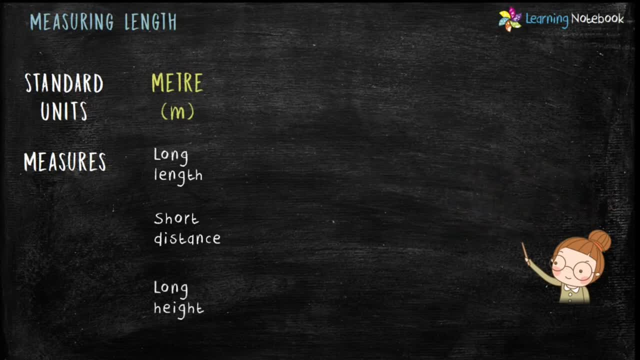 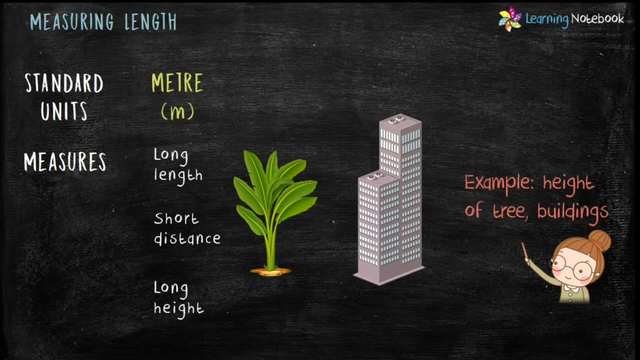 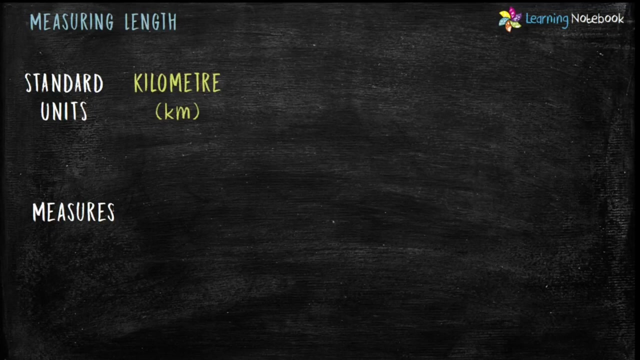 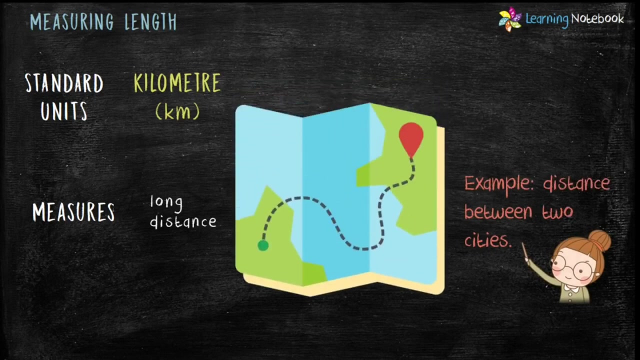 m Students. we also use m to measure long height, For example height of tree or height of buildings. They are measured in m Students. next standard unit to measure length is km. In short, km is written as km. km is used to measure long distance, For example distance. 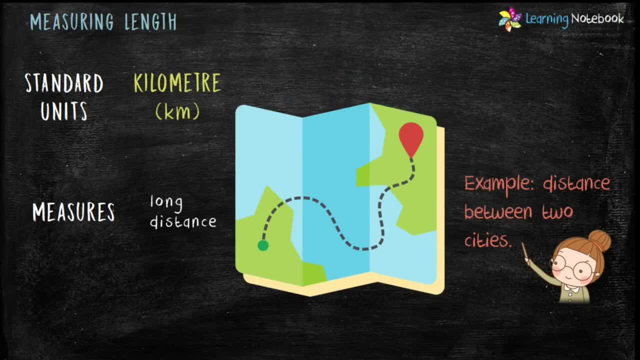 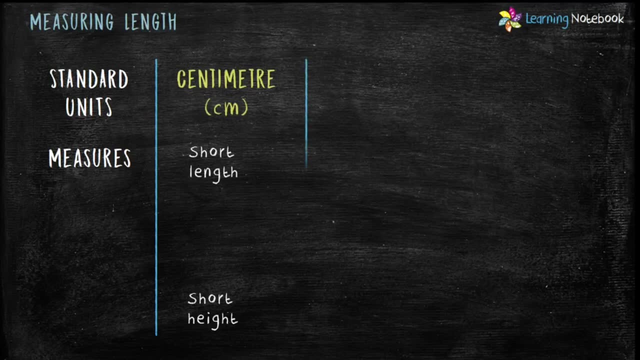 between two cities, For example. distance between two cities, For example, distance between two cities, is always measured in km. So, students, to summarize: cm is used to measure short length and short height. m is used to measure long length, short distance. 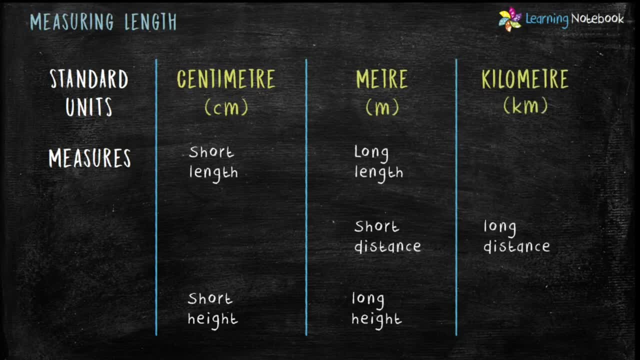 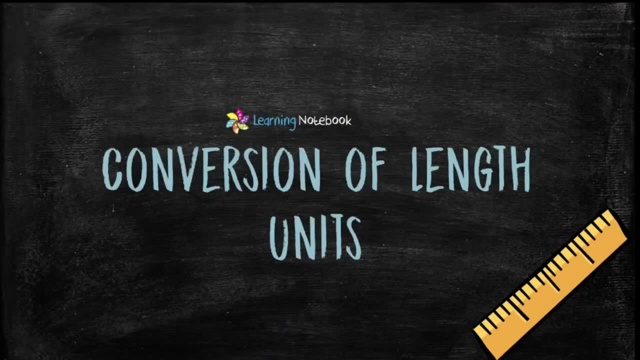 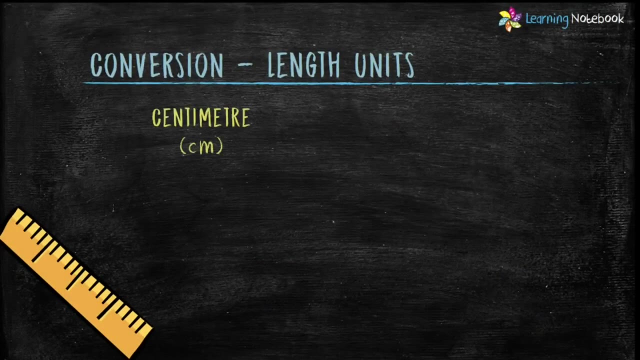 and long height, And km is used to measure only long distance. Now let's see conversion of length units. Till now, we have learnt three standard units of length, which are cm, m and km. Now, students, let's see how to convert km into m and m into cm. 1km equals to 1000 m, So to convert km, 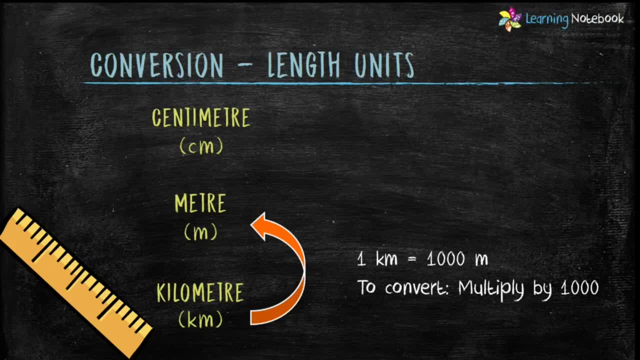 into m, we will multiply by 1000.. So to convert km into m, we will multiply by 1000.. For example, 2 km equals to 2 into 1000, which is equal to 2000 m. Next, 1 m equals to 100 cm. 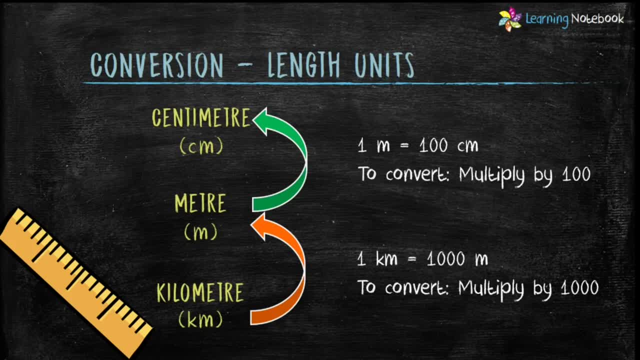 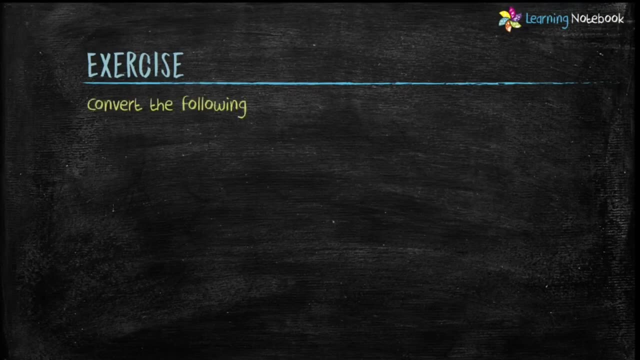 So to convert m into cm, we will multiply by 100. For example, 2 m equals to 2 into 100, which is equal to 200 cm. Now let's do an exercise to understand conversion of length units. First question is: 12 m equals to how many cm? 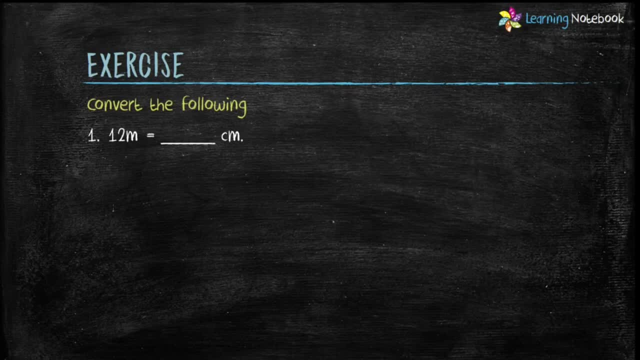 Students, I just told you 1 m equals to 100 cm. So to convert 12 m into cm, we will multiply it by 100 and we get 12 into 100. equals to 1200 cm. Now second part is 9 m. 3 cm equals to how many cm? 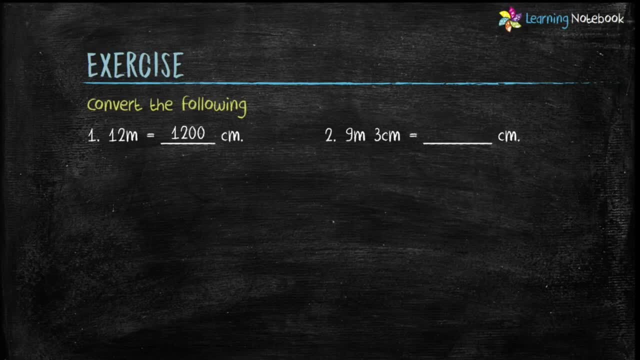 9 m equals to 9 into 100, which is equal to 900 cm. 900 cm plus 3 cm equals to 903 cm. Third part is: 10 m equals to how many cm Students. 1 m equals to 100 cm. 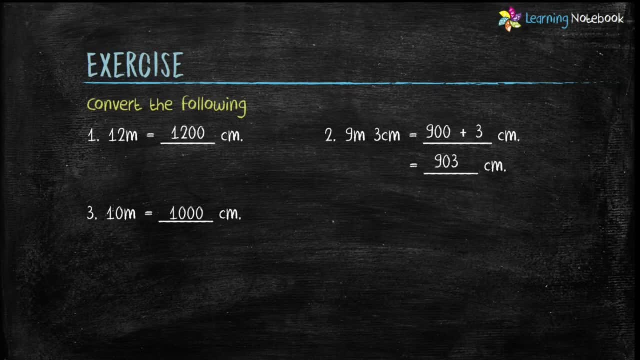 Therefore, 10 m equals to 10 into 100.. Now next one is 6 km equals to 1000 cm. Now next one is 6 km equals to how many m? We know? 1 km equals to 1000 m. 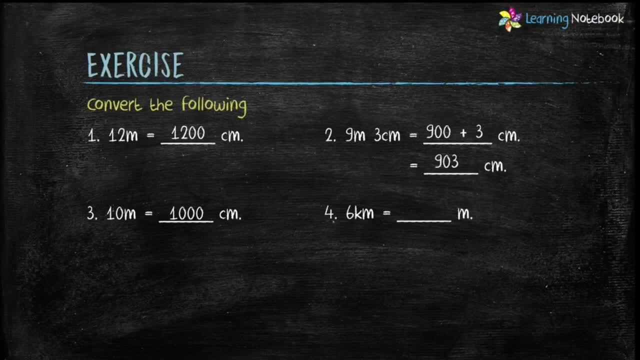 So to convert 6 km into m, we will multiply it by 1000.. Therefore, 6 km equals to 6 into 1000 equals to 6000 m. Now last one is: 7 km equals to 8 into 1000 m. 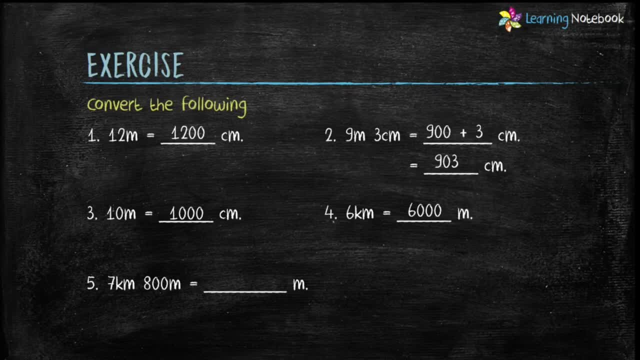 So to convert 7 km into 1000 m, We will multiply it by 1000.. Students: 1 km equals to 1000 m. Therefore 7 km equals to 7 into 1000 equals to 7000 m. 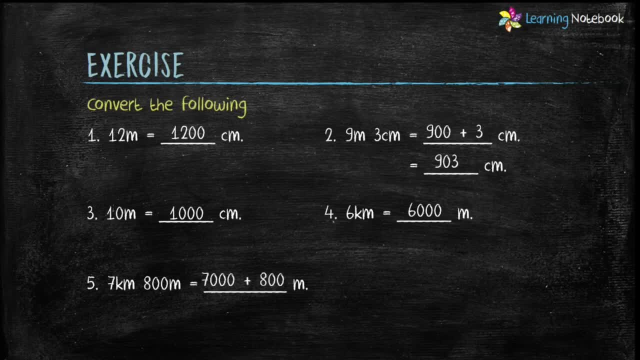 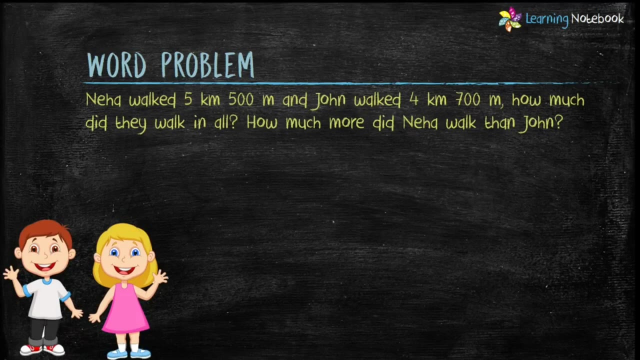 And 7000 m plus 800 m equals to 7800 m. Now let's solve a word problem based on measurement of length units. 1. Neha walked 5 km 500 m and John walked 4 km 700 m. 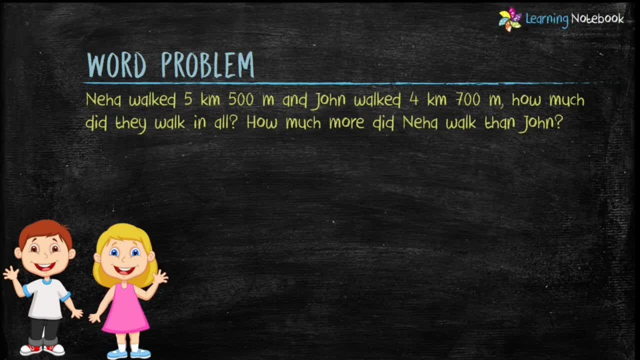 How much did they walk in all? How much more did Neha walk than John? Students always solve word problem with the help of statements. So Neha walked equals to 5 km 500 m. John walked equals to 4 km 700 m. 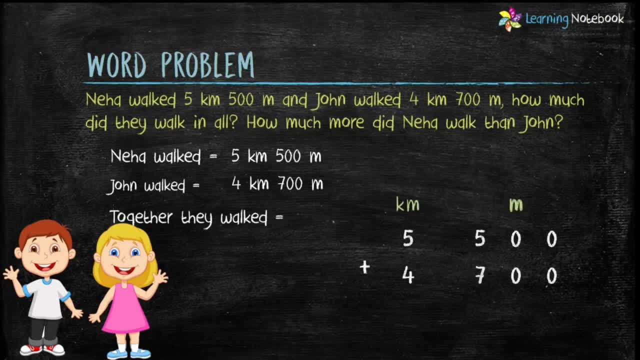 Therefore, together they walked equals to 5 km 500 m plus 4 km 700 m. Write them in columns as shown here. Write meter values below meter unit and write kilometer values below kilometer unit. Now let's add them. 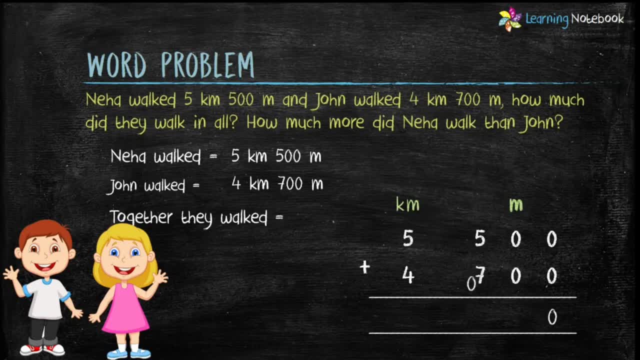 0 plus 0 equals to 0.. Again, 0 plus 0 equals to 0.. 5 plus 7 equals to 7.. 7 equals to 12.. Regroup 12.. 2 comes in the answer and 1 gets carried over. 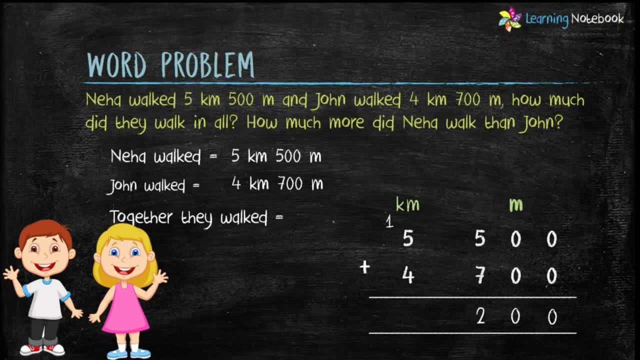 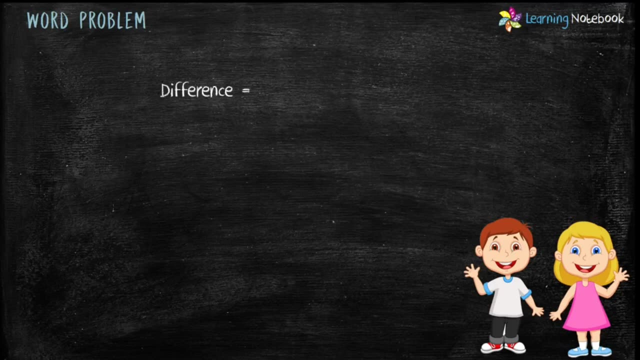 Now, 1 carry plus 5 plus 4 equals to 10.. Therefore, together they walked 10 km, 200 m. Now we have to find how much more did Neha walk than John. So, students, we will find the difference or we will subtract. 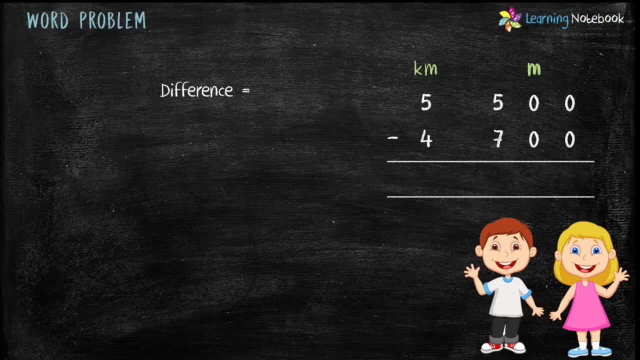 We will write 4 km 700m from 5 km 500m. Write them in columns, as we did while adding: Now let's subtract: 0 minus 0 equals to 0.. Again, 0 minus 0 equals to 0.: 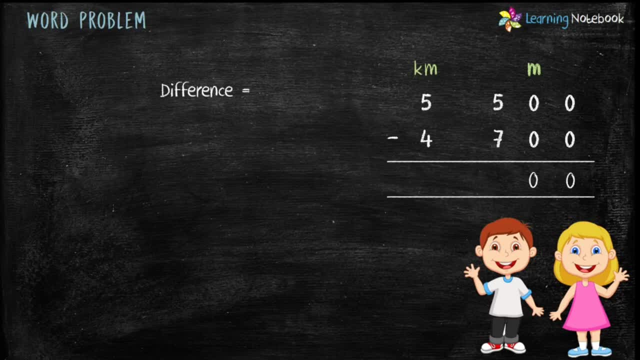 Now, 5 is weaker than 7. So it takes help from its neighbor 5.. Neighbor 5 is kind hearted and give 1 of its power. So neighbor 5 becomes 4 and 5 becomes 2.. 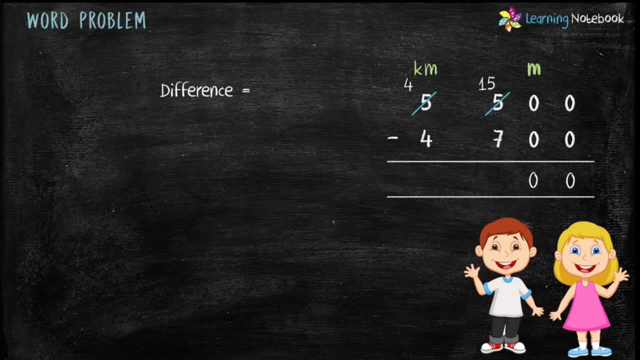 5 becomes 7. and 5 becomes 15. now, 15 minus 7 equals to 8, and 4 minus 4 equals to 0. therefore, they have worked 800 meter more than john. so our answer statement would be: they work 10 kilometer, 200 meter in all.